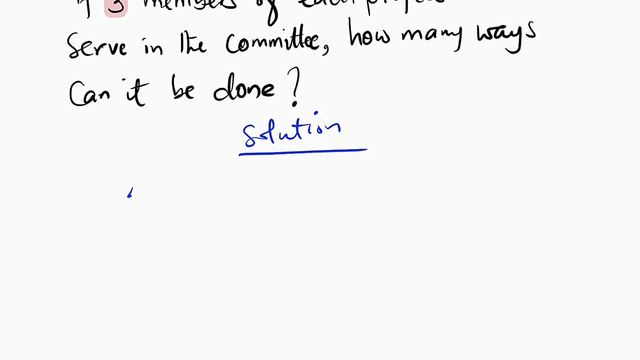 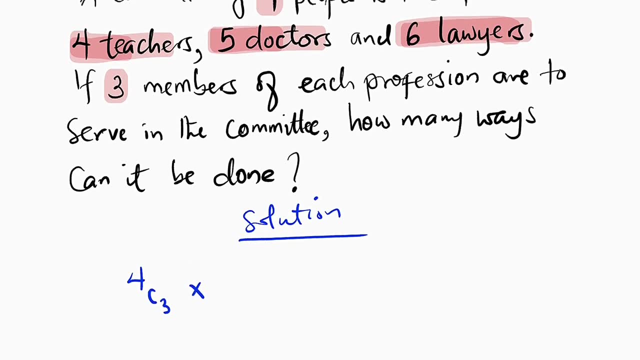 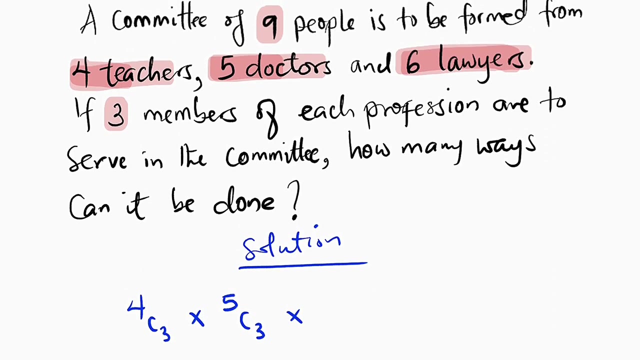 three members from these: four teachers. So we have four, choose three. then we multiply by the second one. We have five doctors and we are going to choose three. So we have five, choose three. then, lastly, we have six lawyers, So we are going to choose three. six, choose three. 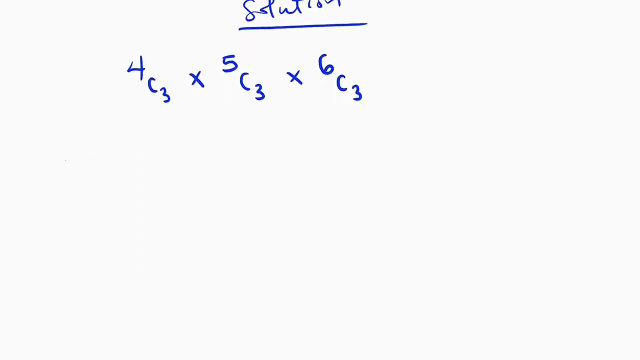 So let's simplify. this is going to be four factorial divided by four minus three factorial, then three factorial, then multiply by five factorial divided by five minus three factorial, divided by three, then 3 factorial. and lastly, multiply by 6 factorial divide by 6 minus 3 factorial, then 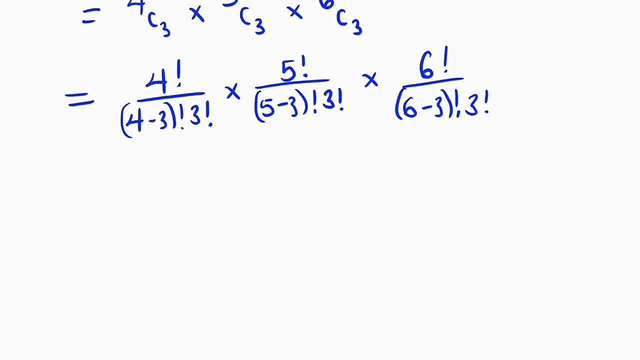 3 factorial. this is equal to 4. factorial divide by 4 minus 3 is 1 factorial, then 3. factorial multiply by 5. factorial divide by 5 minus 3 is 2 factorial, then 3. factorial multiply by 6. factorial divide by 6 minus 3 is 3 factorial, 3 factorial. let's further break it down. 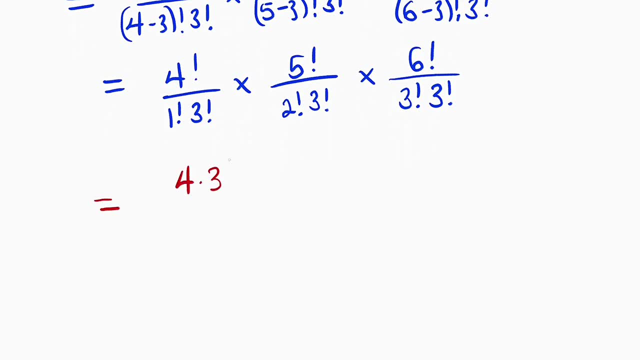 this is equal to 4 multiply by 3 factorial. I will stop here. 1 factorial is one multiplied by three factorial. they are multiplied by five, multiplied by four, multiplied by three factorial, divided by two factorial, or let me write it as two times one they are: 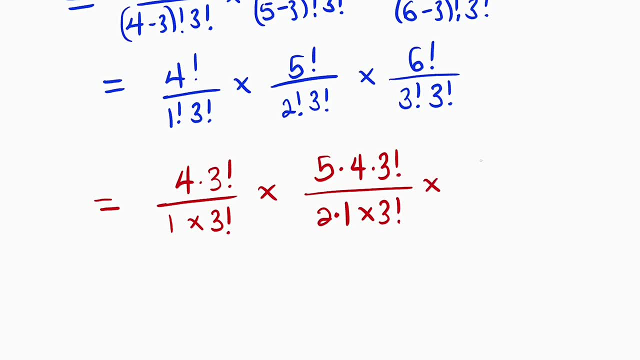 multiplied by three factorial and last one, we have six, five, four, three factorial. I will stop here. let me break three factorial into three times, two times one. then I will leave the other three factorial like this. so, for cancellation, this will cancel this. this will cancel this two times. one is two and it can go into four, two times. so we have three, two, one which is six.